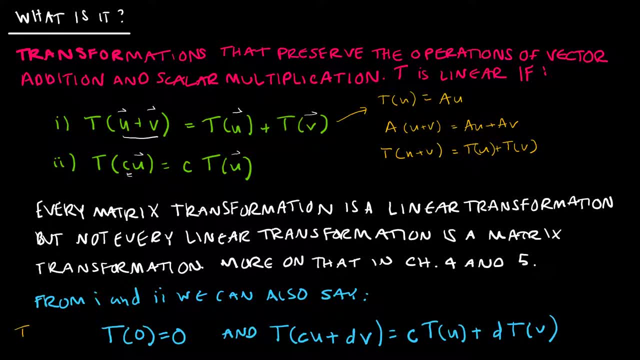 And again, that one's pretty straightforward because it's like T of 0 times U and we can pop it out using this guy and therefore say that of course that's going to be equal to 0.. And then, of course, this one: the transformation of some scalar times a vector plus some scalar times a vector. 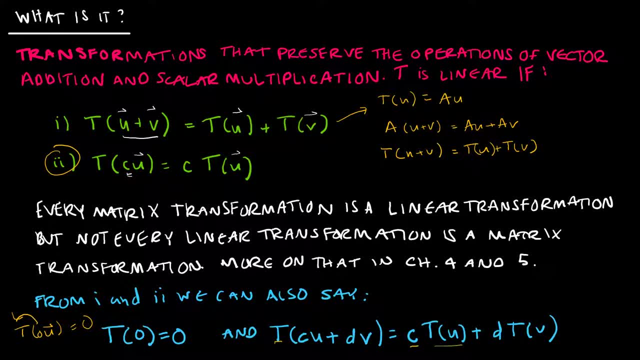 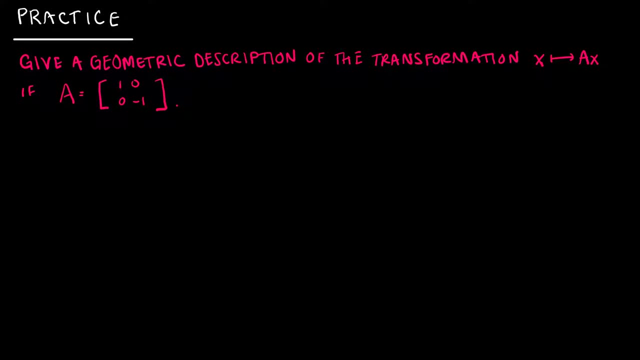 is equal to that: scalar times the first transformation plus the scalar times the second transformation, And again, that's just combining both of those. So why are we learning about this? What kinds of questions are going to be related to linear transformations? Well, quite often we're going to look at the geometric description of these transformations. 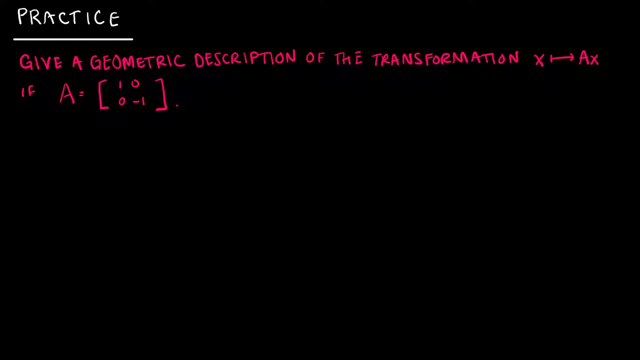 Because we're talking about linear transformations. we can actually see what this is going to look like, So let's start by just drawing in a coordinate plane. Here's my X1 axis and my X2 axis, And I'm just going to stick with very simple values in R2, just so that we can see what they look like. 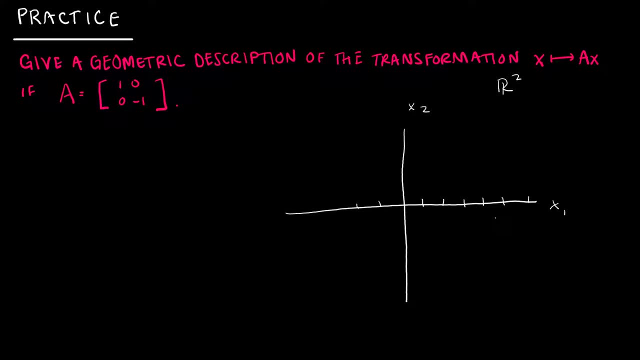 So let's do an example And notice: they haven't changed. They haven't given me any points to look at. But that's okay. All I want to do is see what A is going to do to some vector. So I'm going to make up vector U to be 2, negative 1.. 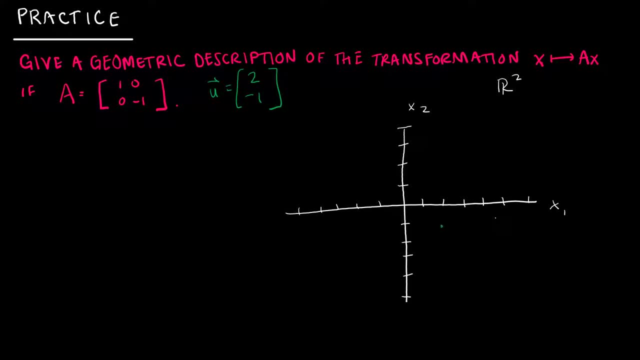 So I've just made it up. You can make up whatever vector you want. So 2, negative 1 looks just like that. That's vector U. What would happen if I take A times U? So let's find out: 1,, 0, 0, negative 1, 2, negative 1.. 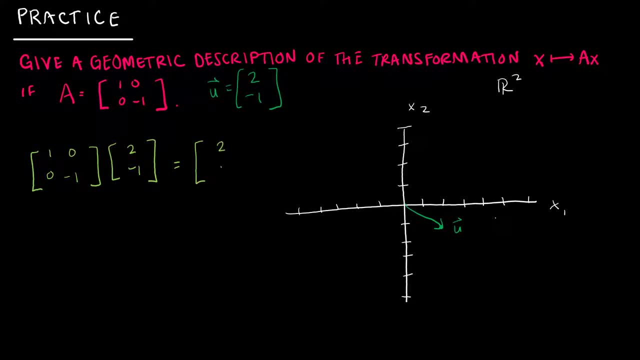 If I do my multiplication, I get 2, positive 1.. So 2, positive 1 is right here. So this is what AU looks like. So what appeared to happen? Well, it looks like I took vector U And I flipped it across the X1 axis. 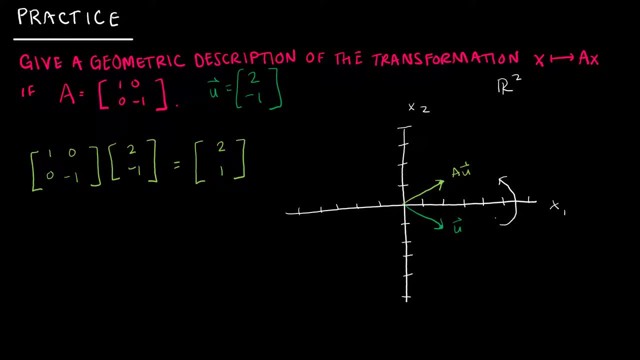 So it appears to be a reflection across X1.. But let's test that theory by trying another one. Let's do vector V. I'll have that be negative 3, 2.. So if I take A times negative 3, 2.. 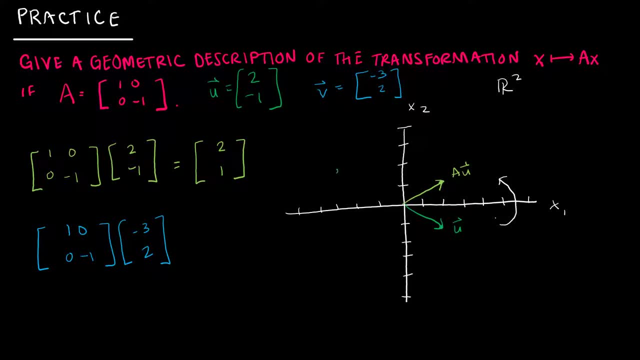 And I should probably go ahead and plot that vector. This is vector V. So what I think is going to happen is it's going to come down here, But let's check it and see what happens. I'm going to get negative 3 and negative 2.. 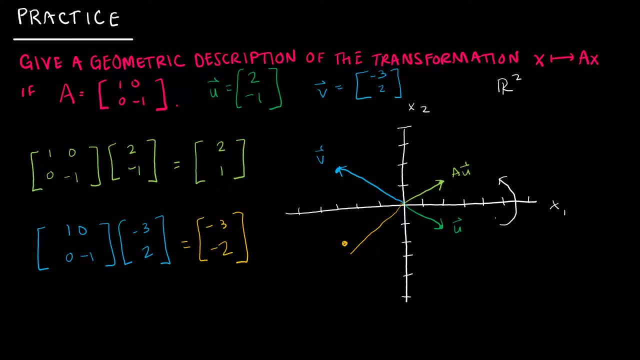 So negative 3,, negative 2,, right there, And it did in fact reflect Across the X1 axis. So what is the geometric description? Let me try again. The geometric description is that this, that A is a reflection across X1.. 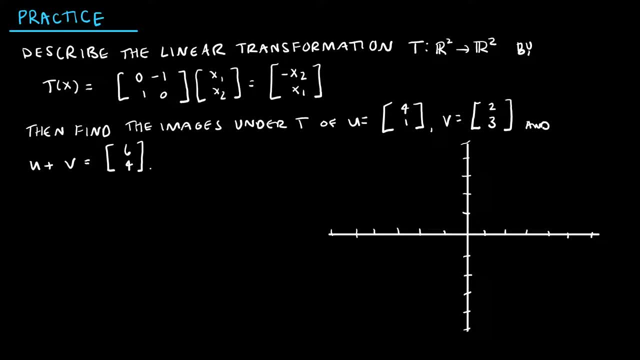 Here's a similar question for you. to try Notice. it's written just a little bit differently. It says: describe the linear transformation T that maps from R2 to R2. By T event. Now, what is this? So what's going to happen? 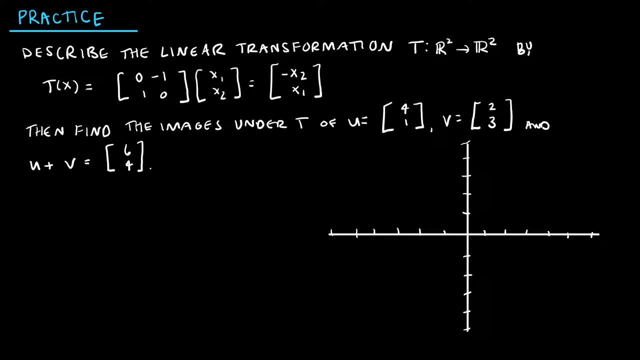 So what I've seen is that the dimension of X is equal to 2. And they've shown me that the A matrix is 0, negative 1, 1, 0. They've already done this multiplication for me, And so really what they've done here is say if you apply T, it's going to swap your X1 and X2 values. 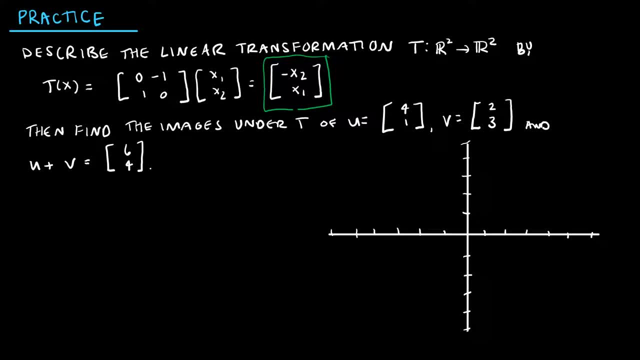 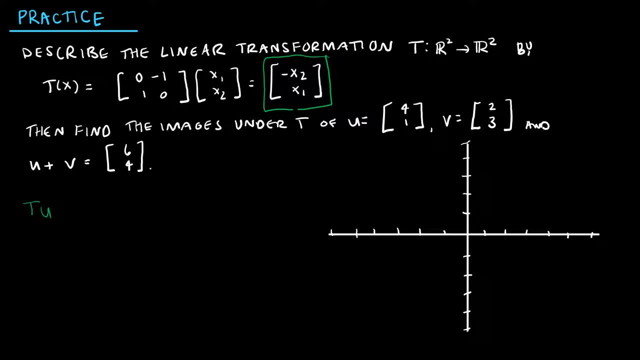 So I can when I'm finding the images of T under images of T, images under T of U. So if I wanted to find T? U, I would be taking 0, negative, 1, 1, 0 times 4, 1.. 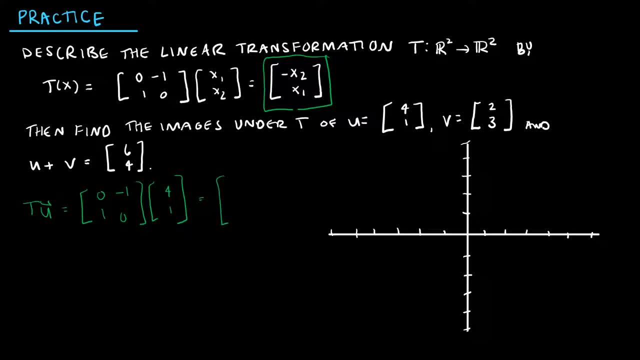 And that would give me negative 1, 4, which I've done by multiplication, the standard way that we've been doing this. So U is 4, 1, and T? U is negative 1, 4.. Now I did that one by normal. 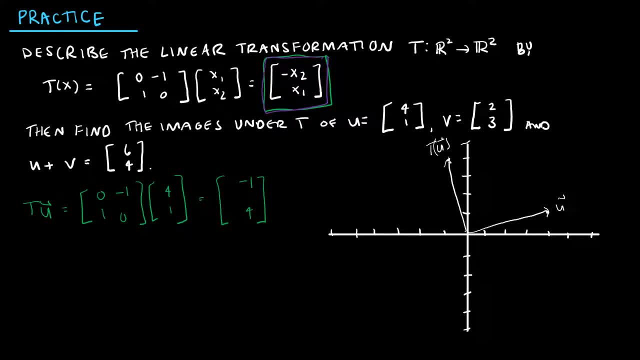 multiplication. but really I can take a look at what they've done here and say if I want to find T V, all I have to do is take V, which is 2, 3, flip them 3, 2, change the sign So V, which is. 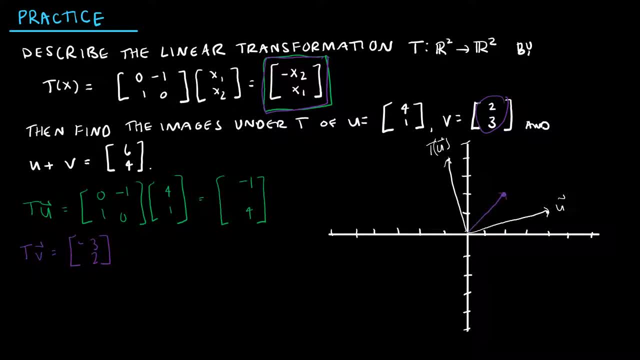 2, 3, becomes negative 3, 2.. So this is negative 3, 2.. T, V And I can do the same for U plus V, which is 6, 4.. So T of U plus V, which is 6, 4, becomes. 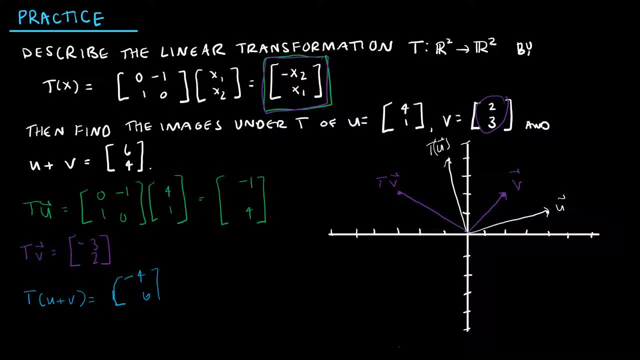 4,, 6.. And change the sign So 6, 4, which, if you'll notice, this is just that parallelogram rule- becomes negative 4,, 1, 2, 3, 4, positive 6,. oops, I don't even have six spaces, We'll. 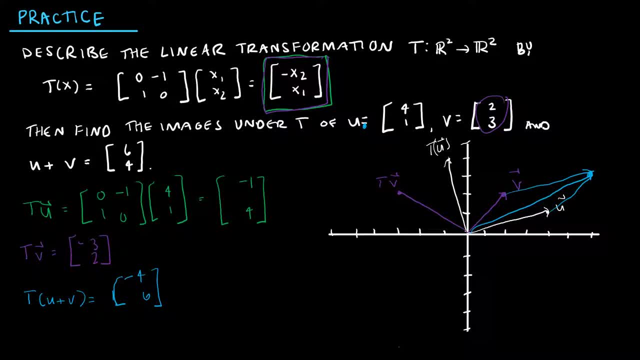 just put it up here. And so again, still parallelogram rule. So what happened to my original parallelogram, which is all over here? this was u plus v, which makes sense because that's what the parallelogram rule says. So what? how? 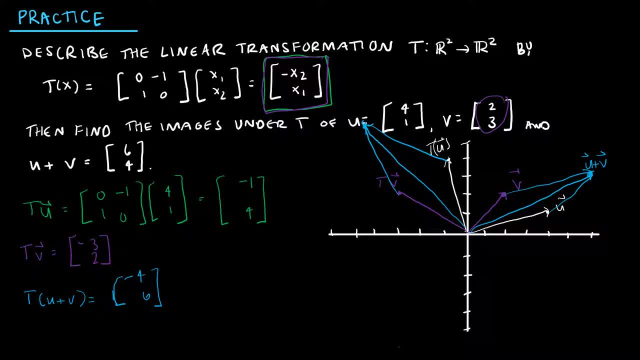 would I describe this linear transformation? Well, it appears that what happened is that I took this figure and I've rotated it, So it wasn't flipped. it was rotated about 90 degrees, counterclockwise about the origin, So this point stayed exactly where it was.